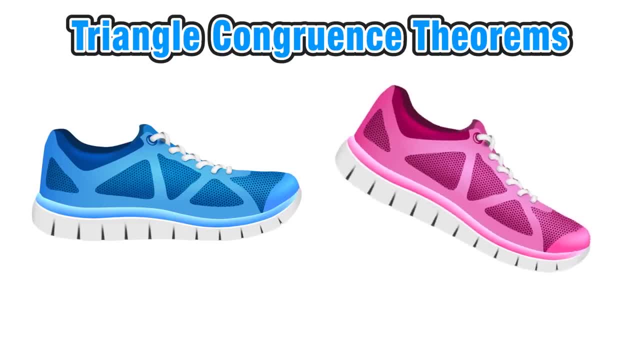 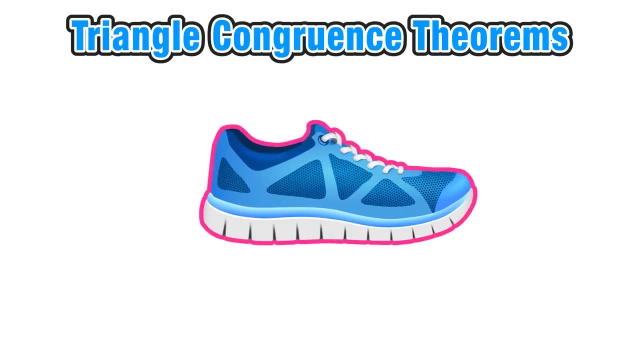 and shape. Now, even if I change the color of one of the shoes or I rotate it around a certain number of degrees, it's still congruent to the original sneaker because it's the same size and shape. And we want to extend this kind of thinking now to comparing triangles to see whether or not. 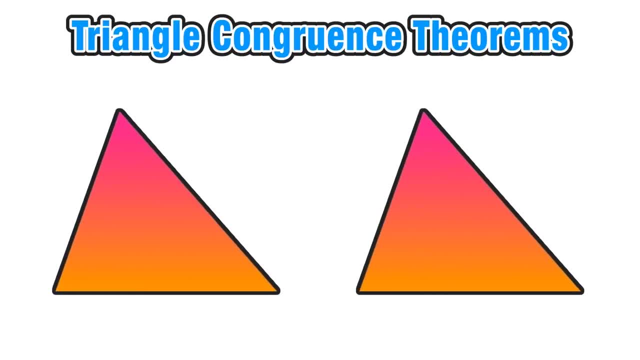 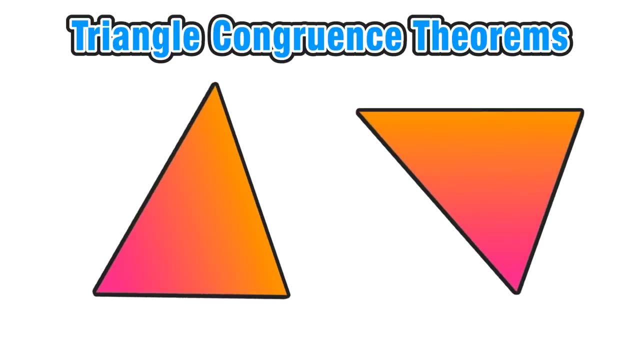 they are congruent. If their corresponding sides and angles have the same measure, then we can say that the triangles are congruent, And this applies even when the figures don't have the same orientation and visually it's not so easy to tell whether or not these triangles are congruent, and this is where our theorems are going. 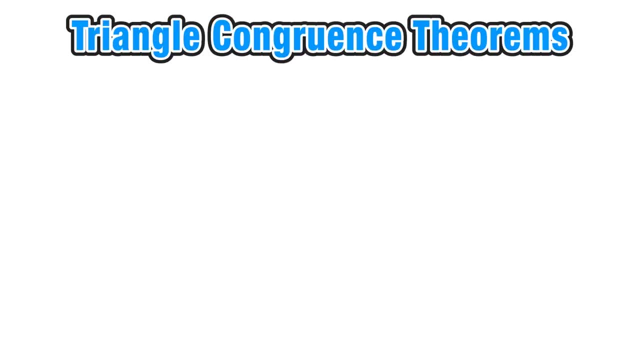 to come into play. So the goal of this lesson is to help you to understand why the theorems that we use prove congruence and how to know which theorem to use in a particular situation. So here are the five triangle theorems with their abbreviations. We have: side-side-side, side-angle-side, 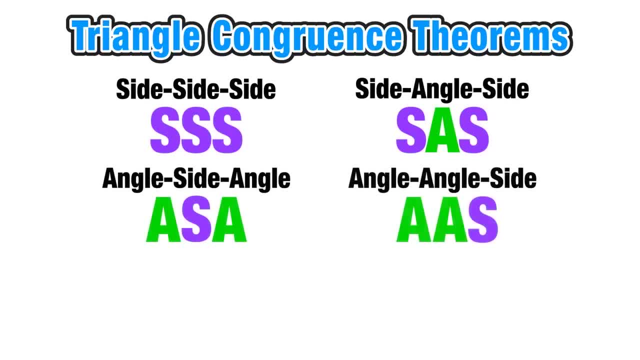 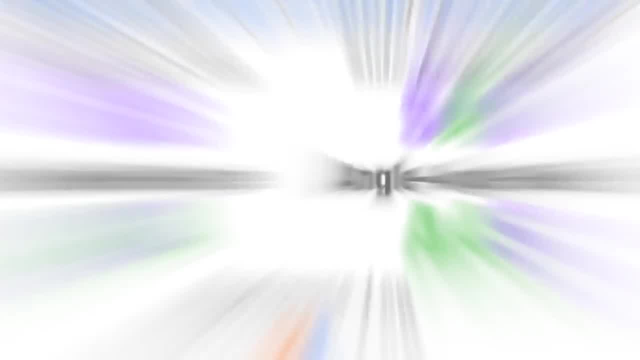 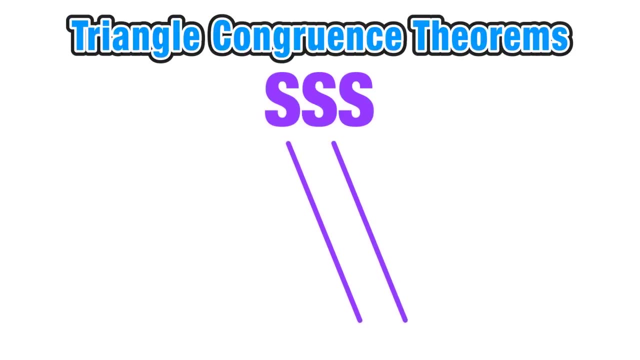 angle-side-angle, angle-angle-side and hypotenuse-leg. So now we're ready to go ahead and explore each theorem individually. Now the side-side-side triangle congruence theorem states that if in two triangles we have three pairs of corresponding sides that are congruent to each, 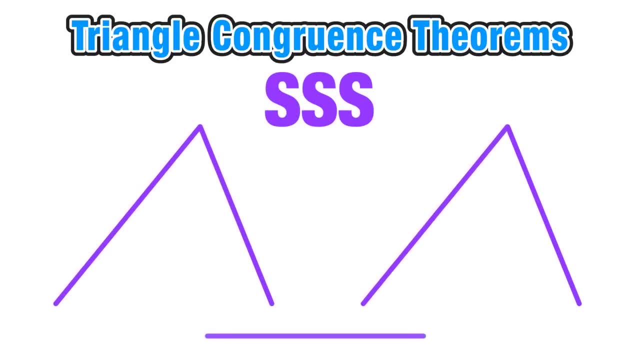 other. that means that they have the same length. then that's enough information to say that the triangles are congruent to each other, Which again just means that both triangles are exactly the same size and shape. So in this instance we can use the side-side-side theorem to conclude that the triangles are 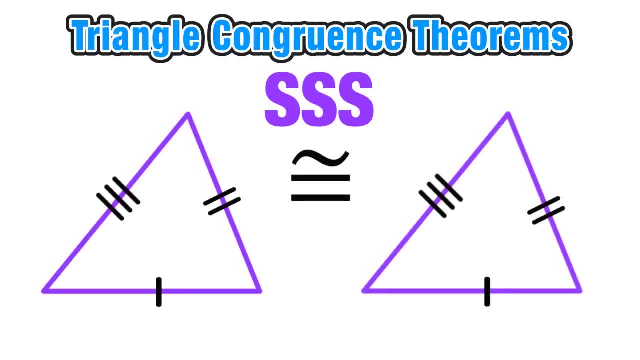 congruent and that their corresponding sides and corresponding angles have the same measure. And remember that this relationship is still true even if the figures have different orientation. Our next theorem is side-angle-side. Now for this triangle congruence theorem. we start with. 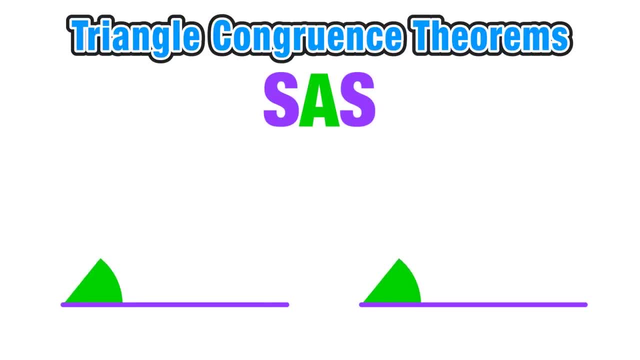 a pair of corresponding congruent sides in two triangles. We also have a pair of corresponding angles that are congruent and another set of corresponding sides that are congruent. Now see that the letter a is in between the two s's in the name of the theorem. 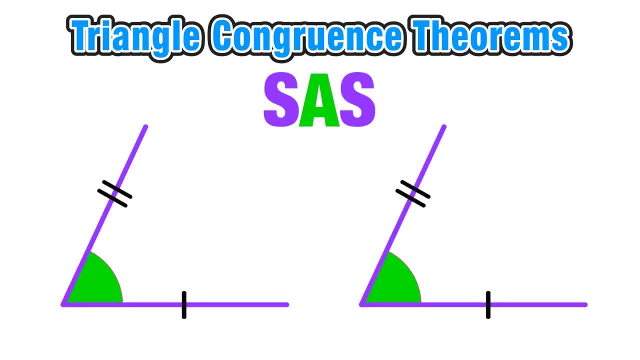 This corresponds with that congruent angle being in between the two congruent sides. Now, in this is the case, we have enough information to say that the two triangles are congruent by using the side-angle-side theorem. Our next congruence theorem is the angle-side-angle theorem. When we have two triangles with a 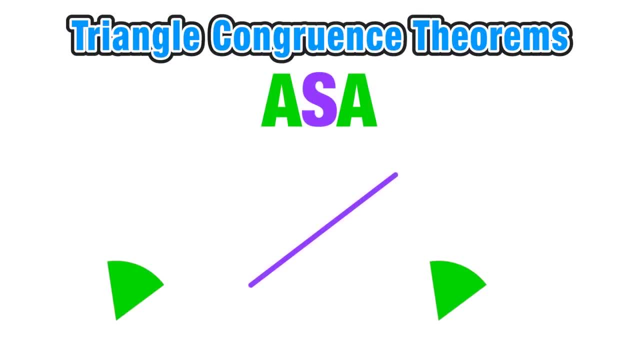 pair of corresponding congruent angles, a pair of corresponding congruent sides and another pair of corresponding congruent angles. we have enough information to prove congruence using angle-side-angle. Now it's important to notice that the congruent side is in between the two congruent angles, And now we can visualize. 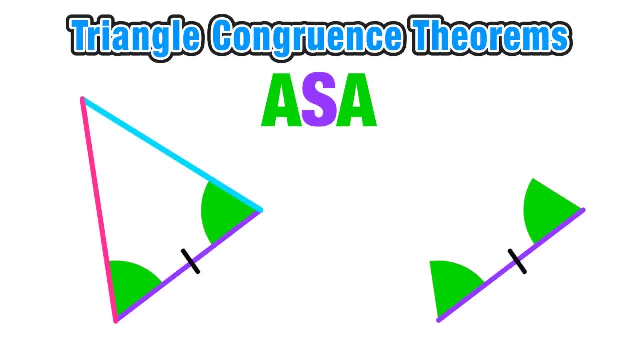 that, when this is the case, we have enough information to prove that the two triangles are congruent by angle-side-angle, which means that all of their corresponding sides and corresponding angles have the same measure. Now our next theorem is very similar to the one. 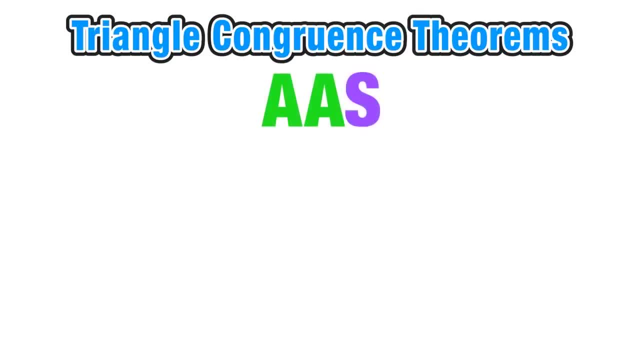 that we just looked at, which was angle-side-angle. This one is called angle-angle-side Now, when, in two triangles, we have a pair of corresponding congruent angles, along with a second pair of corresponding congruent angles, as well as a pair of corresponding congruent sides. Now we don't. 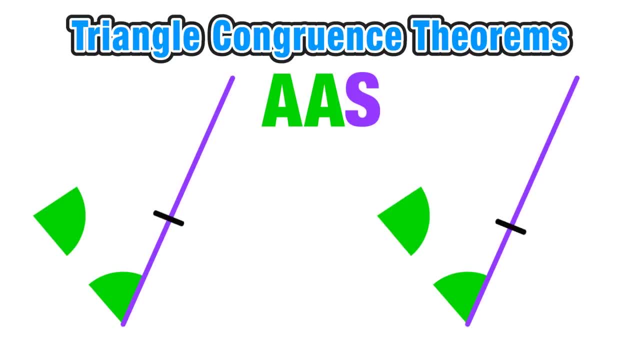 want to confuse the last theorem, angle-side-angle, with the second pair of corresponding congruent angles and this theorem of angle-angle-side, because both of them involve two congruent angles and one congruent side. The difference is that in angle-angle-side, the congruent 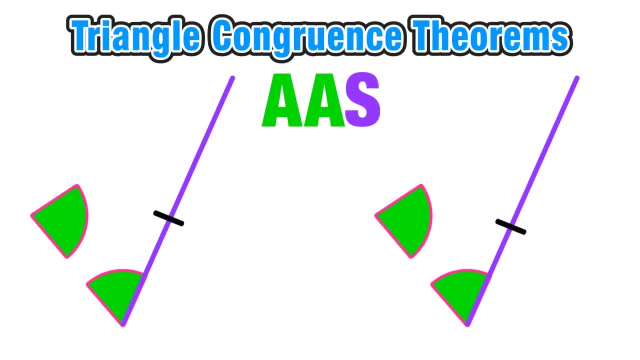 angles are consecutive, that is that they are one after the other, And then the congruent side is next to them instead of in between them. Now, even though the order is different, we still have enough information here to prove that these two triangles are congruent, which. 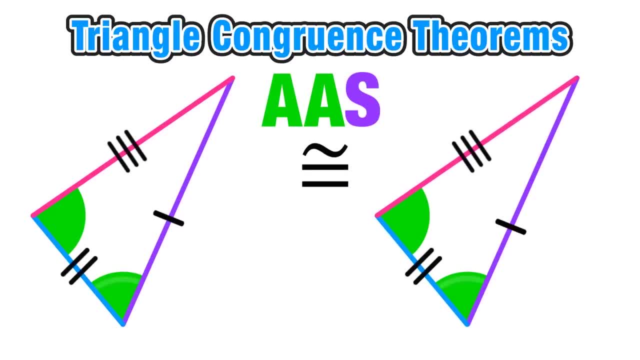 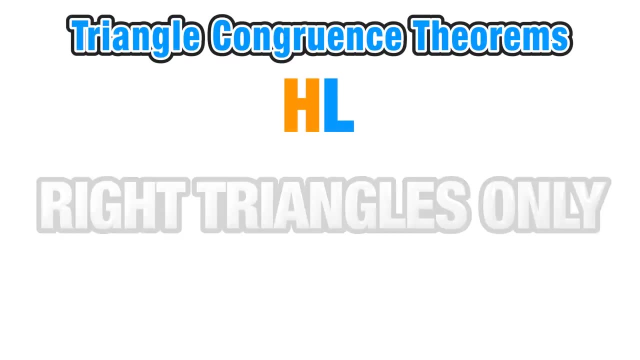 means again that they're congruent. Now our final congruence theorem is kind of a special case. it's called hypotenuse leg and it applies to right triangles only. So let's start out with the key feature of any right triangle, and that is a right angle.